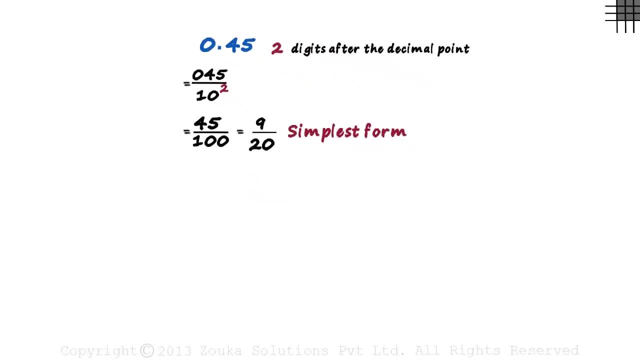 of digits after the decimal point. Here's another example: 2.225.. It has 3 digits after the decimal point. So first we write the number without the decimal point, It will be 2225. And divide it by 10 raised to 3.. We write 3 as the power of 10, since 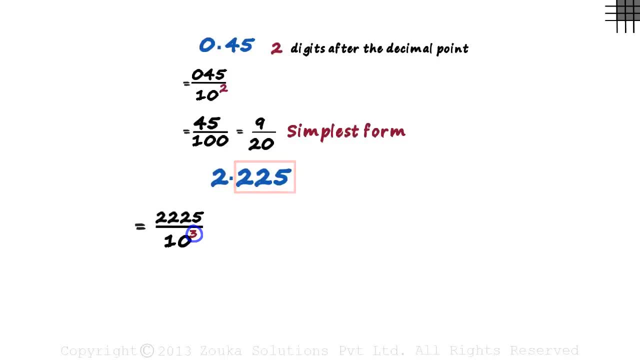 we have 3 digits after the decimal point And that will equal 2225 by 1000. And this can be reduced to 89 by 40. So we wrote 2.225 as 89 by 40. That was simple. But what if? 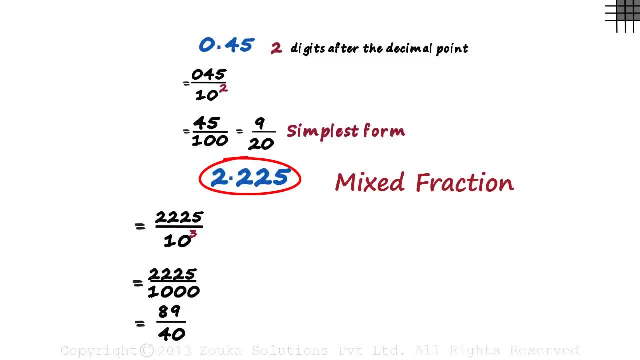 you're asked to write 2.225 as 89 by 40?? You can write 2.225 as 89 by 40.. That was simple. But what if you're asked to write 2.225 as a mixed fraction? A mixed fraction. 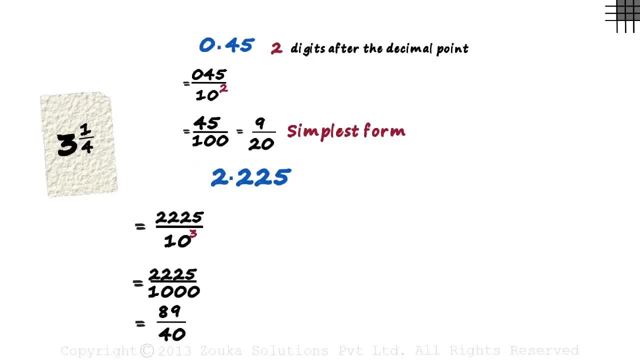 is something like 3, one by 4.. It means 3 and a quarter. Three is called the whole part and one by 4 is called the fractional part. So how do we get this decimal form in this mixed fraction form? It's very simple. The whole part is the number to the left of the 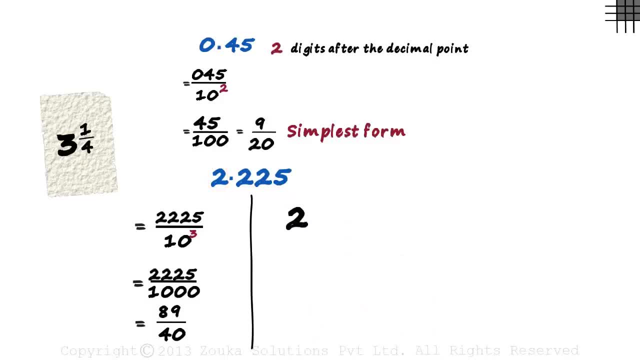 decimal point Two becomes the whole part. The numerator of the fractional part is the number to the right of the decimal point. it's 225.. And guess what? The denominator of the fractional part is the same as the denominator in the previous case: 10 raised. 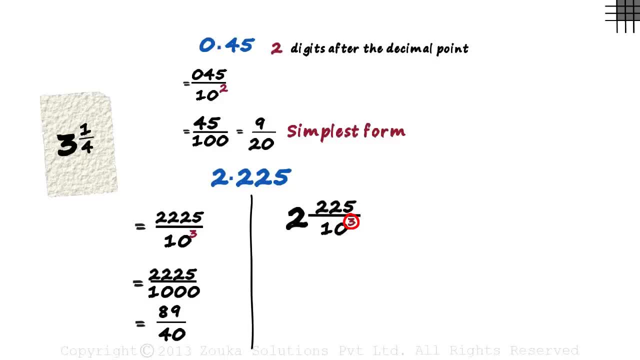 to 3.. Again, the power of 10 is equal to the number of digits after the decimal point. That's it. Now we just have to simplify the fractional part to its simplest form. This can be written as 2 225 by 1000.. This is the whole part and this is the fractional. 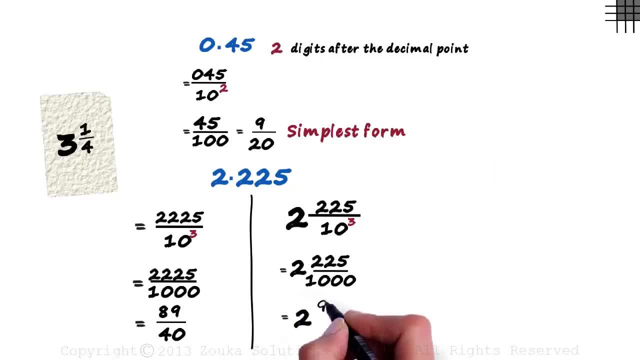 part. This, when reduced, gives us 9 by 40. So 2.225 can be written as 2, 9 by 40. That becomes our mixed fraction form. Just to check your answer, it's always recommended that you convert this into a normal fraction and verify. This would equal 2 multiplied by 40. 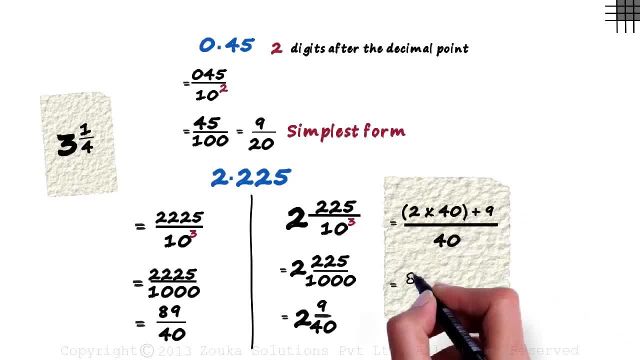 plus 9 by 40. That would equal 80 plus 9 by 40, which equals 89 by 40. Same as the answer we got earlier. While converting it into a mixed fraction, just remember that the number to the left of the decimal will be the whole part and the number to the right of the decimal